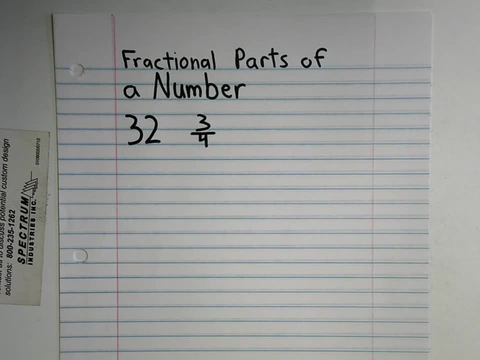 to know what is three fourths of 32? now I'm going to show you how to do it using a picture first. okay, now three fourths. which number is my denominator? which number is my denominator, Josh? for the number on the bottom, that's how many total parts we have in all. so what I'm going to do, 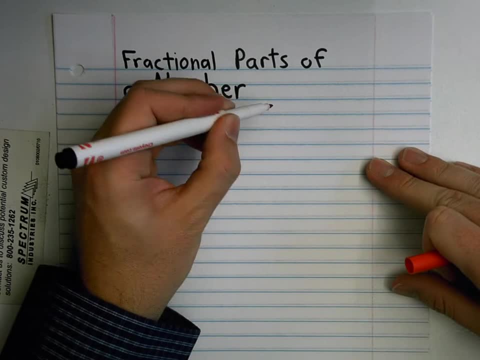 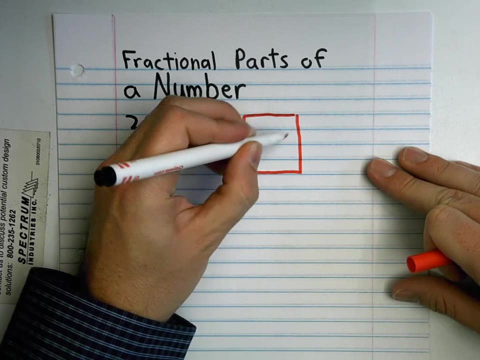 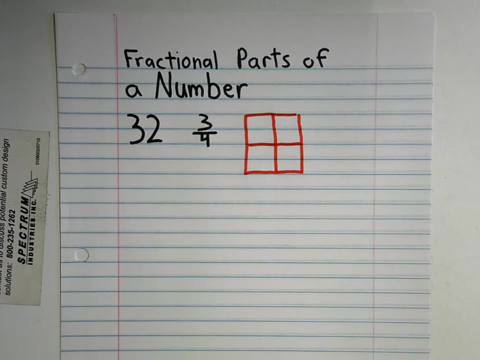 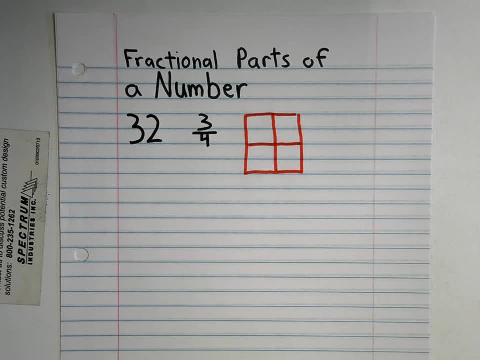 doing numbers. well, I can use this picture to show us how to do the numbers and then, when I show you just the way, using the numbers, it'll, it'll make sense. okay, now, how many pieces do I have? I have 32, don't I? in four parts. let's go, I'm gonna do. I'm gonna split up these 32 pieces among four. 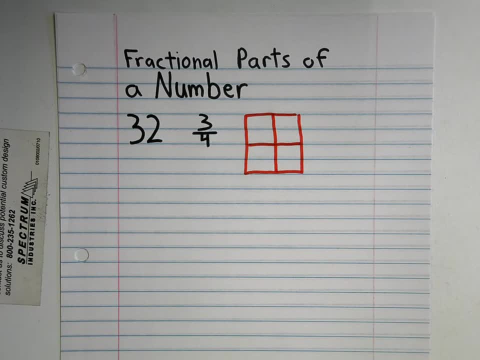 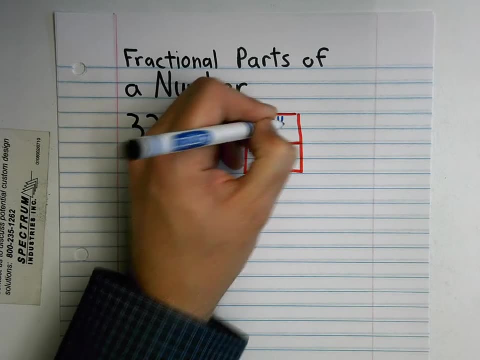 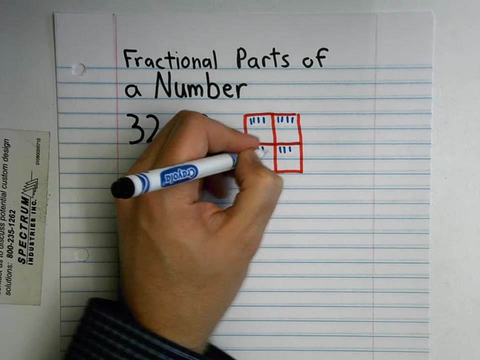 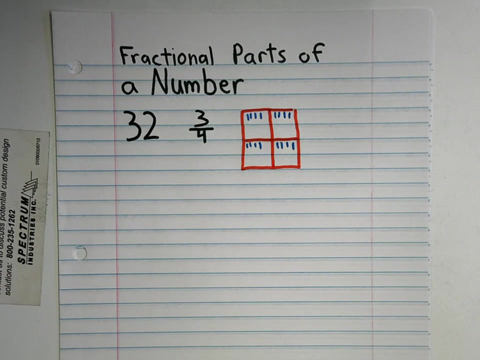 parts equally. okay, kind of like we're doing division, because basically a fraction is a division problem. okay, so one, two, three, four, five, six, seven, eight, nine, ten, eleven, twelve, thirteen, fourteen, fifteen, sixteen. why am I putting them in one square at a time? Logan, yeah, that way I'm making sure I 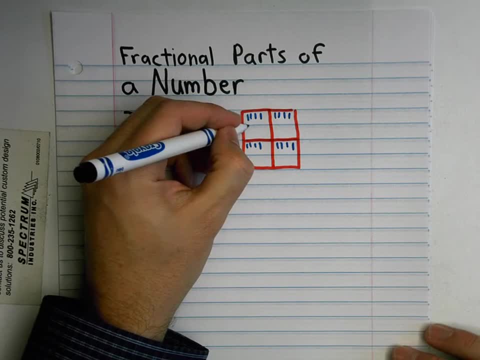 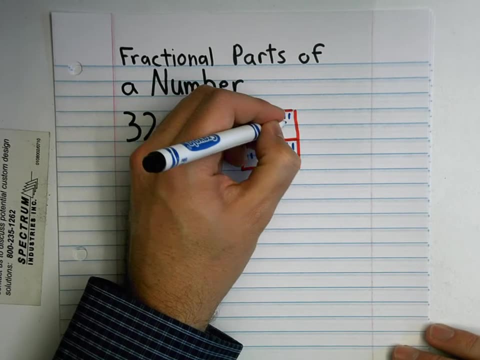 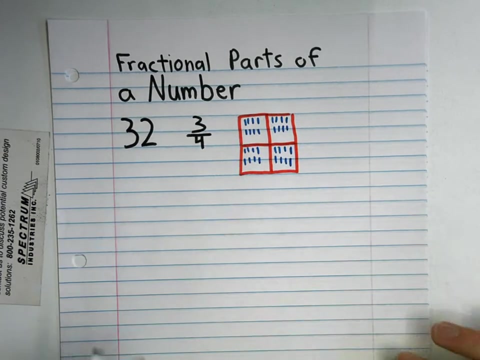 have the same amount in each one. they're even good, good, good call: 17, 18, 19, 20, 21, 22, 23, 24, 25, 26, 27, 28, 23,, 24,, 25,, 26,, 27,, 28,, 29,, 30,, 31,, 32.. 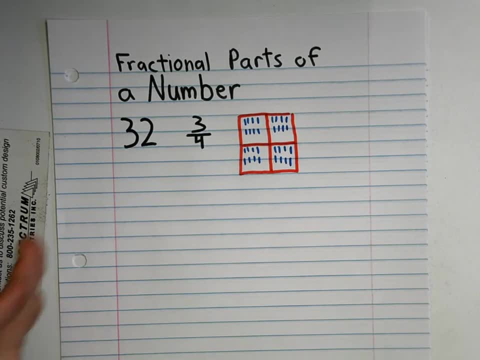 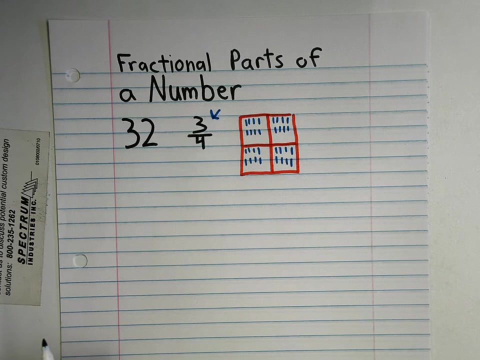 Now, how many do I have in each box in each of my four parts? 10.. Eight, I have eight, But it's asking for three of those. So how many are there in three of those boxes? Hmm, Blake. 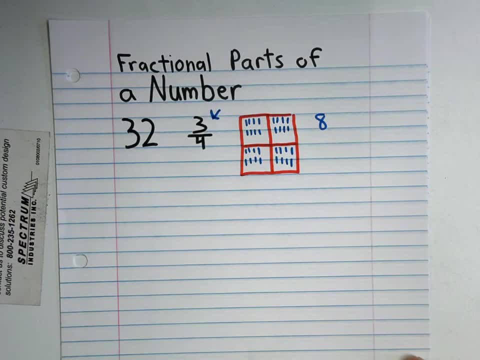 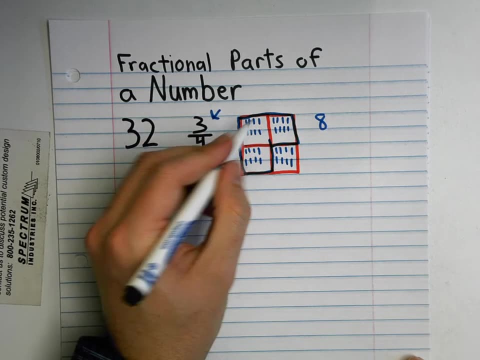 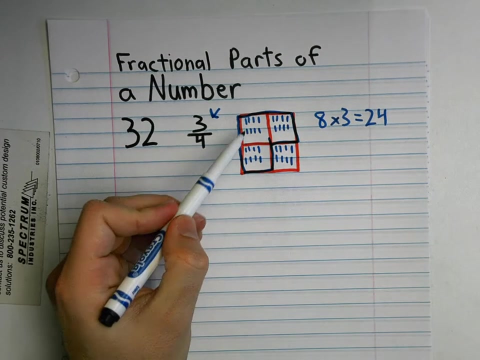 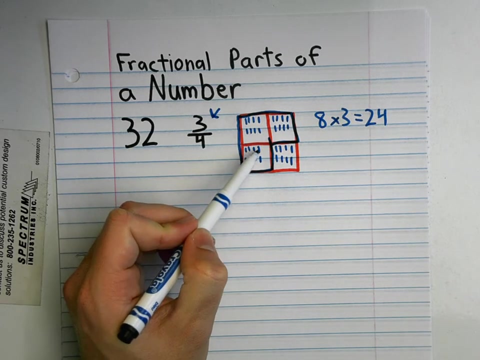 24.. Because, look, I take my eight and I multiply it by the three boxes, I'm going to count, and there's times, 3 equals 24.. I'll count just to make sure, OK: 1, 2,, 3,, 4,, 5,, 6,, 7,, 8,, 9,, 10,, 11,, 12,, 13,, 14,, 15,, 16,, 17,, 18,. 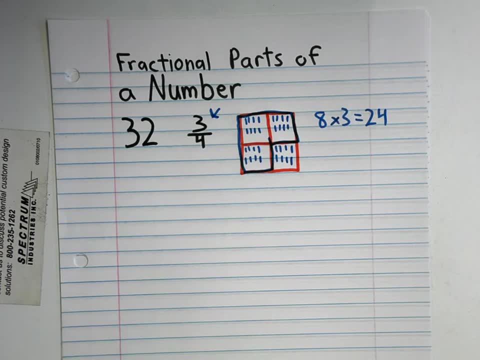 19,, 20,, 21,, 22,, 23,, 24. 24.. So 3 fourths of 32.. I drew it out, put the numbers in the right boxes and found out that it was 24.. 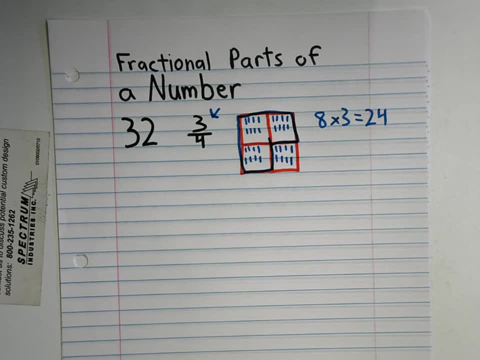 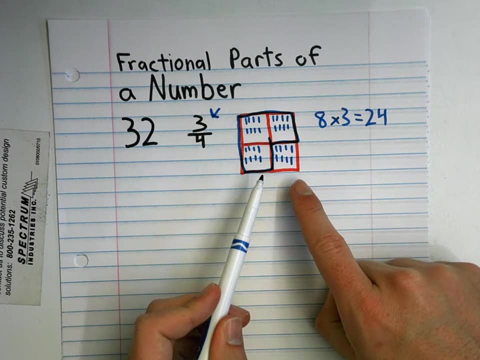 But I want to think of something we did here. Didn't we just take this 32, and the first thing we did, didn't we divide it into four equal parts? We divided it by the denominator, didn't we? Then what did we do? 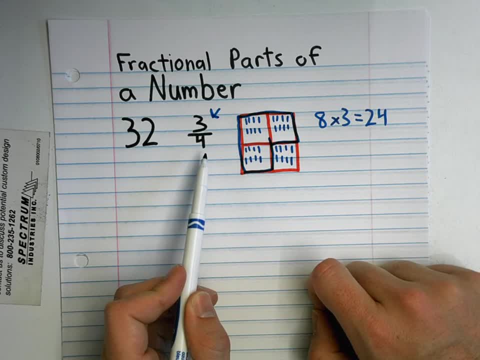 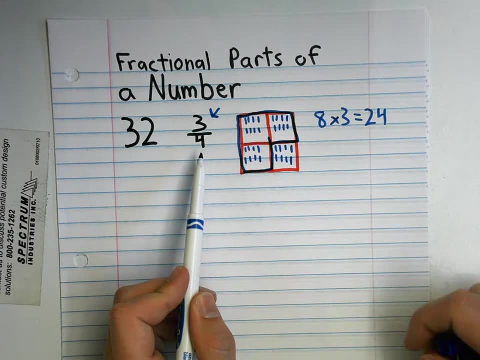 Josh, Josh, Josh, Josh Josh. You separated 32 into four equal parts. Yeah, I did that. first I divided it into four equal parts, So I divided it by the denominator. Then what did I do? Multiplied it by 3.. 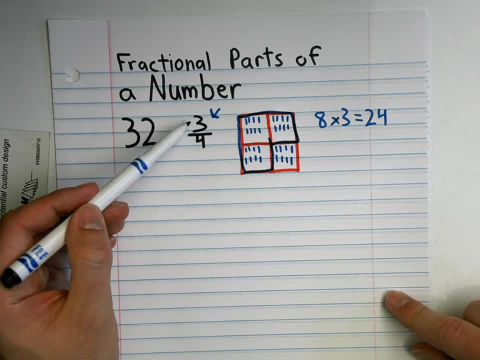 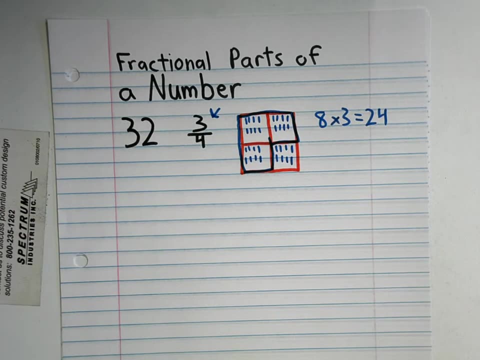 And what's 3?? 3 is the? what's that number on the top called The numerator Nathan? Good job. So basically, when I have one of these, what I do is I divide it by the denominator Denominator and multiply it by the numerator. 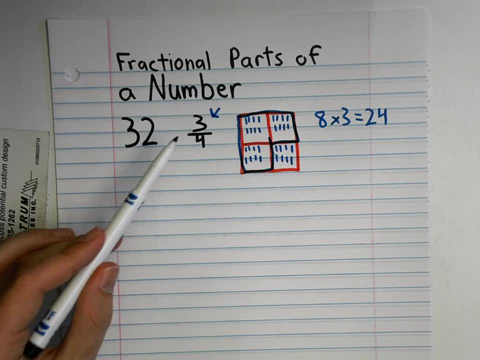 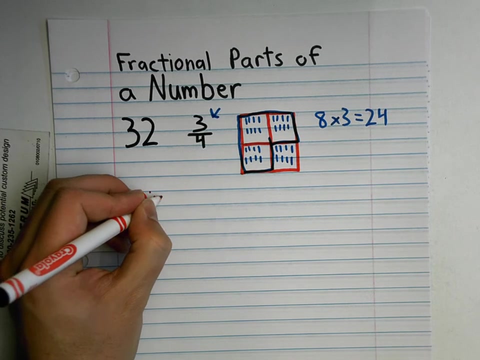 Now it doesn't matter which order. I could have gone. 32 times 3,. then divide it by 4. It'll probably be harder, It'll be bigger numbers, But watch what I can do. Step one: divide by the denominator.